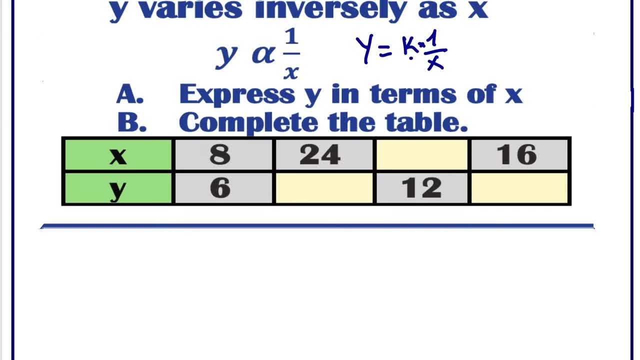 variation. Next, we can go further to say: 1 times k is k. This implies y equals to k over x. Our first question is to express y in terms of x, So it means we should write a formula that has y and x. Okay, 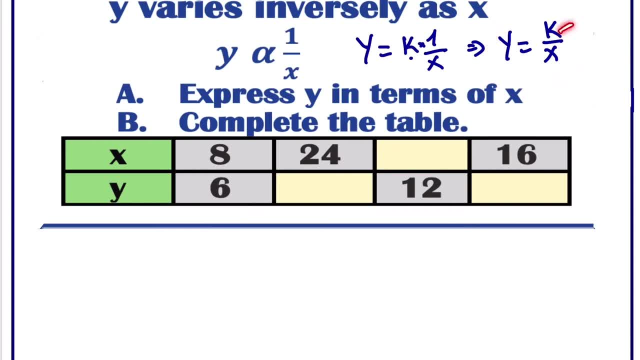 Follow me So in this, so we can see that we have k here. k is the constant of proportionality, of variation, The variation constant. we need to look for k. So, in order to look for k, we have to look carefully at the table where x and y is given so that we can substitute. 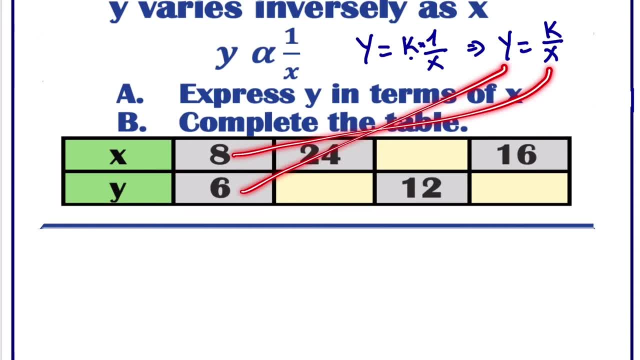 the value of x, the value of y. This will enable us to get the value of k. So first step, let's rewrite the formula. first, y is equal to y, y equals to k over x. So here x, y is 6.. So I write: 6 equals to k over x is 8.. So if 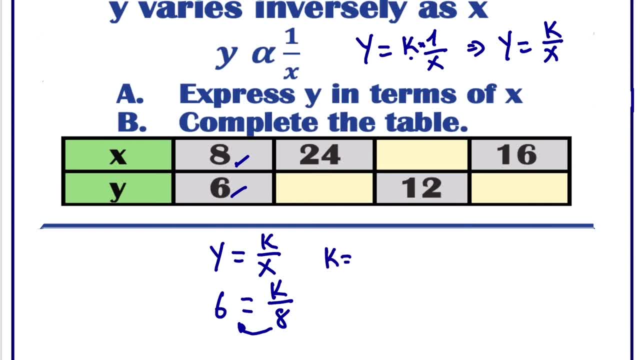 we cross multiply, we are going to have: k will be equals to 6 times 8.. k will be equals to 48.. So this is the value of k. Now that we have the value of k, to write the formula of express y in terms of x, we just block in the value here. So this will be: y will be. 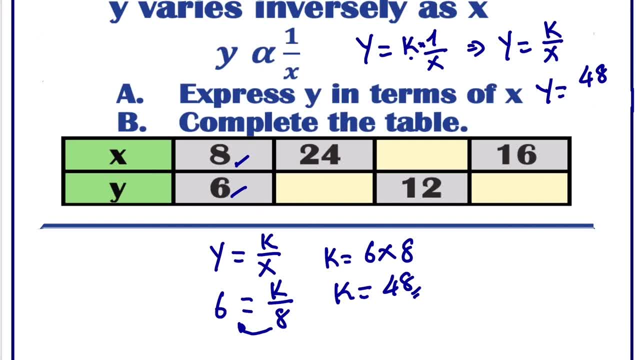 equals to k is 48.. 48 over x. So we can see we have y in terms of x. The next thing to do is to complete the table. In order to complete this table, make sure that you write the formula, because the formula is going to help you. 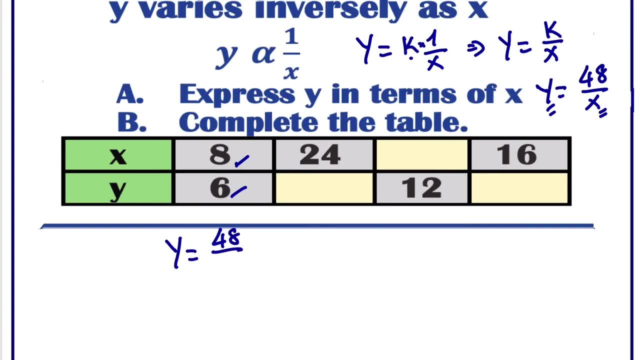 y equals to x, y equals to 48 over x. So to complete this table, we can see here: x was given, x was given, y is not given. So we just need to block in the value of x in the given place. 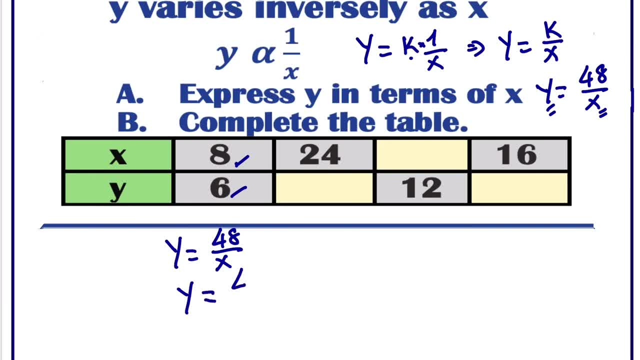 So y will be equals to 48 over x. x here is 24.. So 48 divided by 24, y will be equals to 42. So we can complete it here. We have 2.. Next, still by using the formula here: